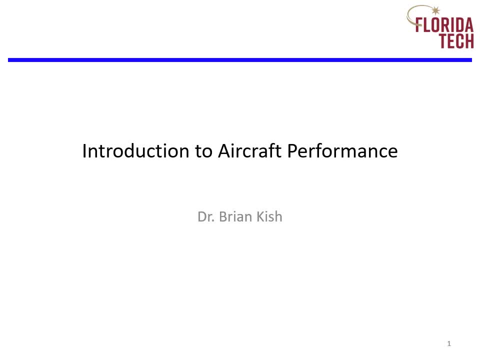 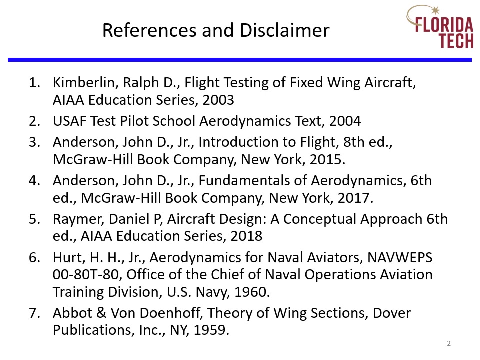 the designer must make decisions regarding wing size, power plant selection, airfoil selection, wing shape and many, many other considerations. All of these help to tailor the design to give the aircraft the desired performance characteristics. There are many references for aircraft performance. I've listed the main ones used in building the material. 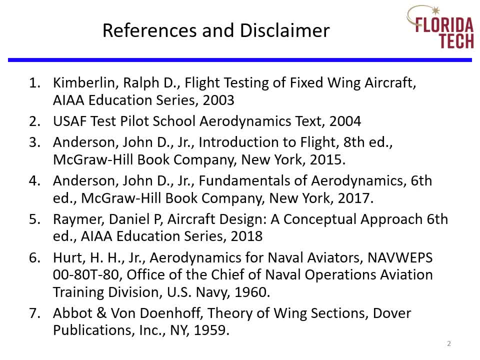 for this course. I've also used pictures and diagrams found on the internet. Since Florida Tech's primary mission is to educate students, we are authorized as faculty members to use other people's work for educational purposes. While we try to document sources as much as possible, we are actually allowed to use information without documenting the sources. 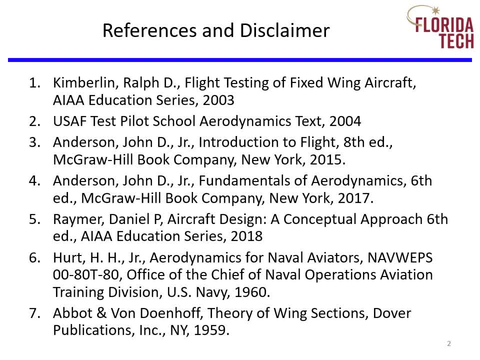 for lectures, So please don't bring me up on plagiarism charges. When it comes to material paid for by US tax dollars, which is the case for US Air Force and Navy test pilot schools, as well as the military academies, the material is assumed. 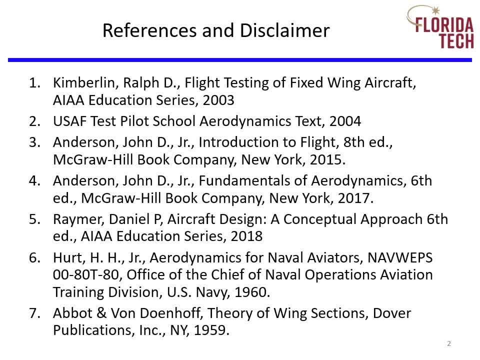 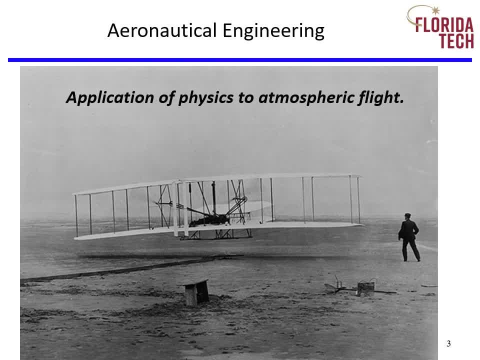 to be public domain. Aeronautical engineering is the application of physics to atmospheric flight For convenience. aeronautical engineering can be arbitrarily divided between two fields. These are into several interrelated sub-disciplines. Note that aircraft performance is just one of these sub-disciplines and is 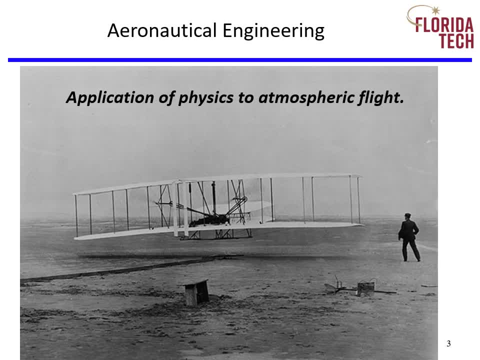 particularly concerned with dynamics: the study of forces, energy and motion. Specifically, performance looks at how an aircraft climbs, accelerates or maneuvers to successfully accomplish a mission. Modern methods analyze and evaluate how effectively an aircraft gains or loses mechanical energy. Terms like agility and 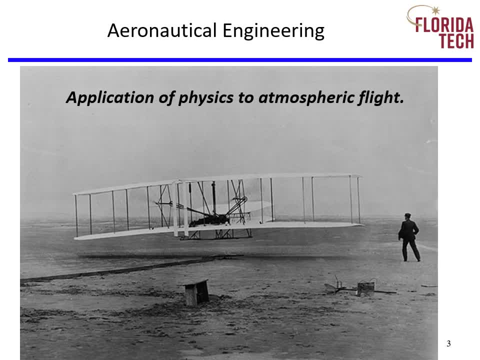 energy maneuvering describe managing aircraft energy state rather than managing trajectory. Once specific models describing forces and motion for flight vehicles have been developed, they can be examined to identify aircraft features which are important in design, testing and operations. This understanding sharpens intuition about how aircraft behavior. 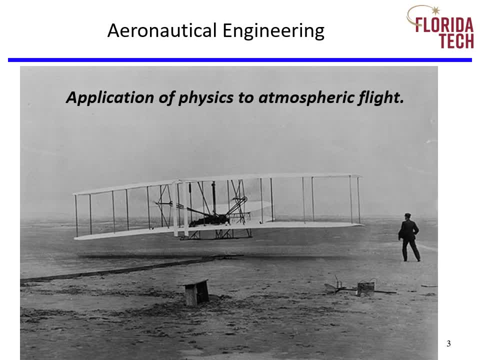 and develops competence in describing aircraft motion. Both are essential, even for those who are not aeronautical engineers, To success in flight tests. we need both for planning and execution and in communicating test results to designers, engineers and operators, who are the end users of results of that. 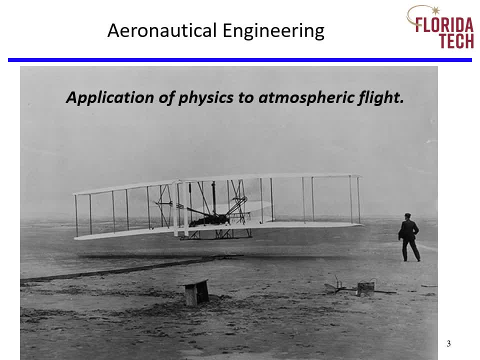 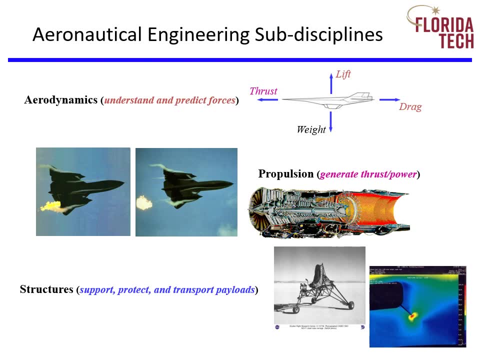 testing. We'll break down aeronautical engineering into eight sub-disciplines. The goal of aerodynamics is to understand and predict lift and drag. Propulsion is how we generate thrust or power. And structures involves how we support, protect and. 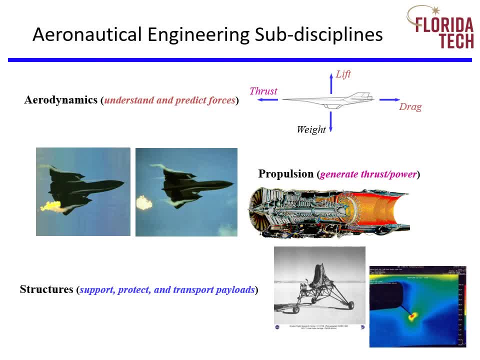 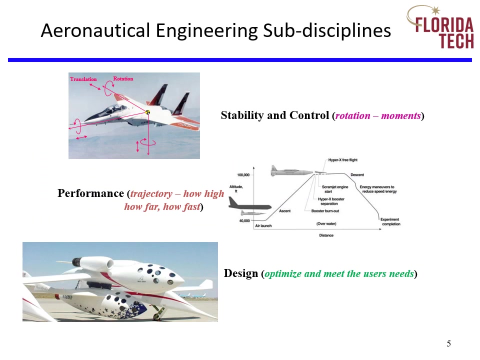 transport payloads. There are full undergraduate college courses for each of these sub-disciplines. We'll cover the highlights of aerodynamics and propulsion in this course. structures, however, will not be reviewed, Although performance and stability control are similar topics- in fact they are often- 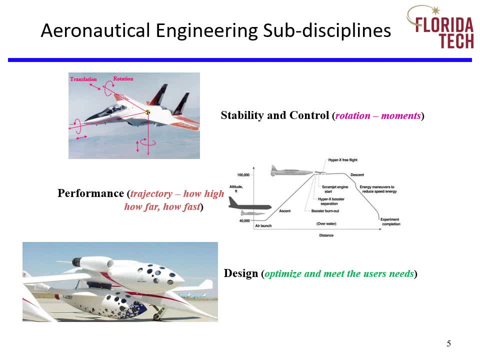 grouped together and called flight sciences. They, however, do have some significant differences. Performance is the study of forces acting on the aircraft and how those forces affect aircraft trajectory. Performance takes a far away view and usually looks at the aircraft as a point mass. 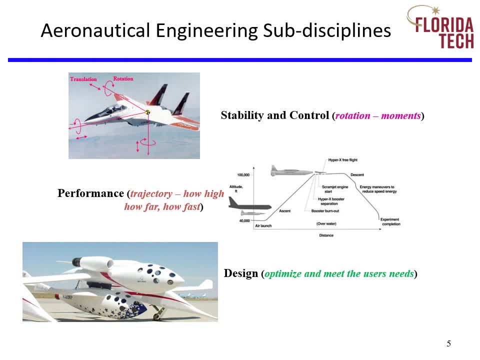 Aircraft, orientation and point of application of individual forces are usually not relevant. In contrast, stability and control is a close-up view of the aircraft. The primary concerns are the moments acting on the aircraft and how those moments affect rotation and orientation of the aircraft. 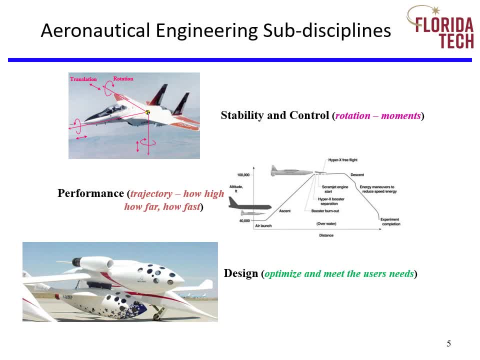 Forces and their points of application are interesting only as they create moments. Performance and stability control are generally unconcerned with how forces and moments are created. They simply assume the forces and moments are known. Aerodynamics and propulsion, on the other hand, are concerned with understanding how. 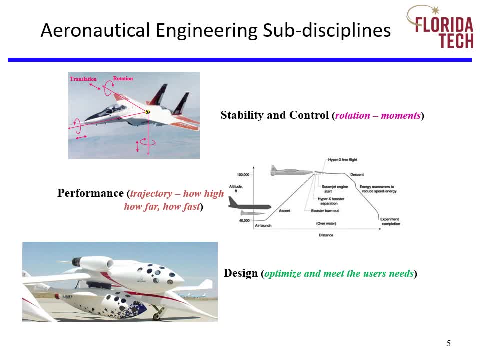 forces are created and predicting those forces. Although aerodynamics, propulsion and stability control are generally unconcerned with how forces and moments are created, they are often coupled by the fact that the aircraft and engine may produce forces when the aircraft changes its orientation. 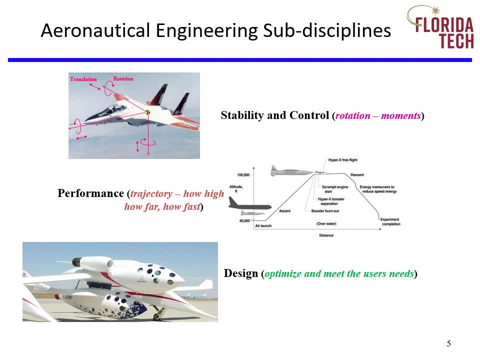 Performance can be subdivided into steady-state performance and dynamic performance. Steady-state performance considers forces in equilibrium or quasi-equilibrium. In this case, velocity and other flight patterns are different, The forces and moments are different. This means those forces in equilibrium and 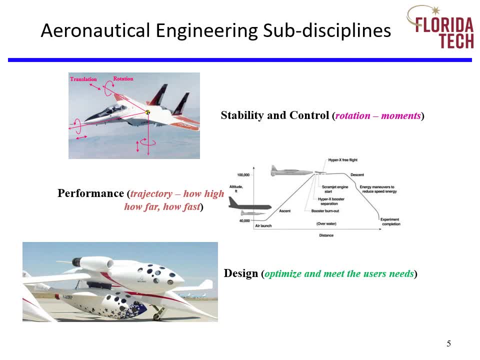 fast- Motor and acceleration can't be mycket cores considered along with the basic parameters which describe steady-state performance. Performance requirements originate with aircraft users. Performance is a primary consideration in the sale of an aircraft to the individual owner, an airline or the military. 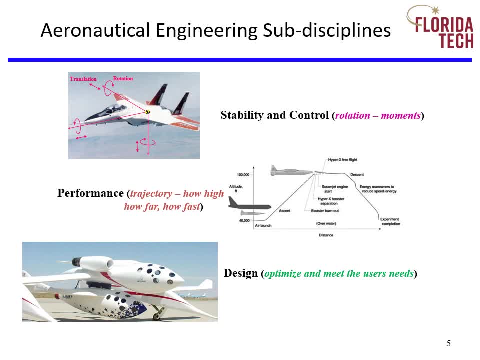 An individual aircraft owner purchases an aircraft to meet specific needs for range, takeoff distance, payload and cruise speed. Airliners must have sufficient range, payload and cruise performance to produce revenue and must satisfy FAA minimum performance requirements to be certified to carry passengers or cargo. 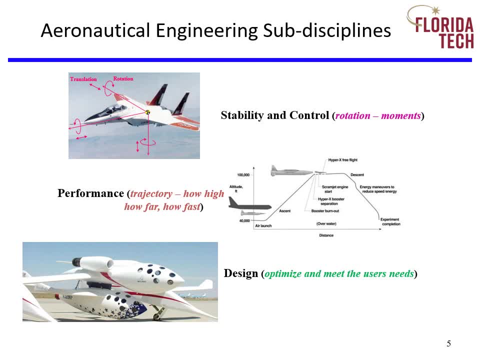 In the military using command, specify performance requirements that provide an operational capability to perform a mission. Buying an airplane implies an expensive business transaction and the buyer will be very concerned that his or her specifications are met. Aircraft operators must accurately describe the performance goals they want the aircraft 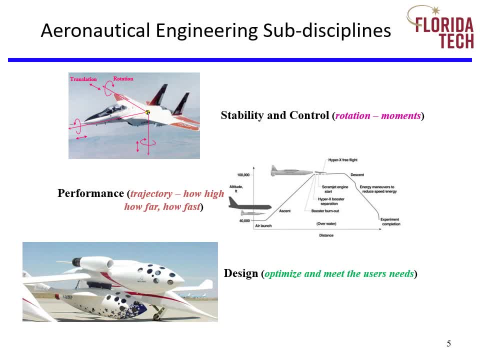 to meet. Contractors and flight testers must accurately describe aircraft performance so the operator or the buyer can determine if his or her goals have been met. If a new aircraft is designed and developed, the contractor specifies performance guarantees. The contractors are normally required to perform a mission and the buyer is required to perform. 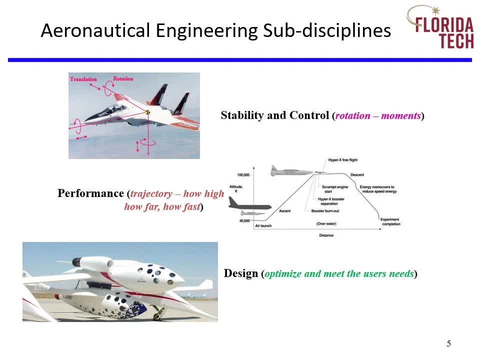 a mission and the buyer is required to provide complete estimates of aircraft performance in performance consistent with flight manual and performance data charts. Designers make decisions regarding aircraft shape and engine selection to achieve airframe performance and operational characteristics described by the customer. These decisions must be integrated and optimized to achieve performance and cost goals, and 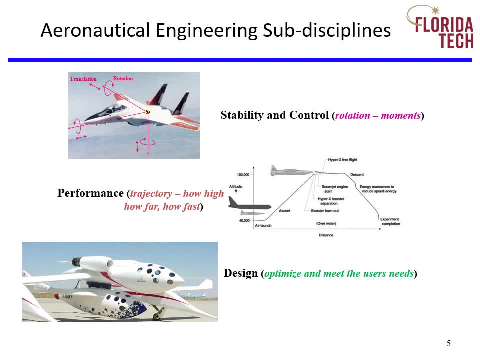 every decision has a profound impact on what the aircraft looks like, how it performs and how much it costs, as well as how well it flies as it performs its mission. Optimizing an aircraft design requires extensive use of aerodynamic and propulsion software models to predict performance. 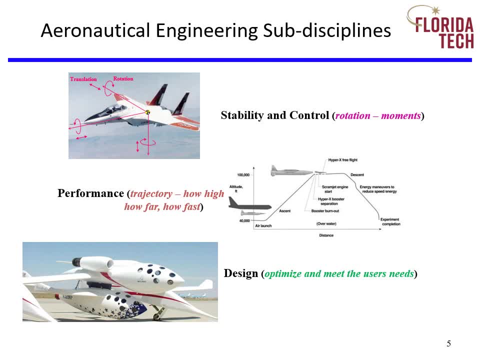 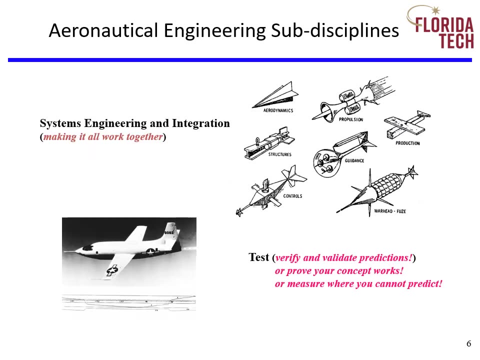 Aerodynamic models are relationships between lift, drag and angle of attack. Propulsion models predict thrust or power and fuel consumption as functions of flight condition and control settings. Aircraft performance may also be defined as the ability of the aircraft to carry a payload in a particular speed, altitude and maneuver envelope over a particular distance. 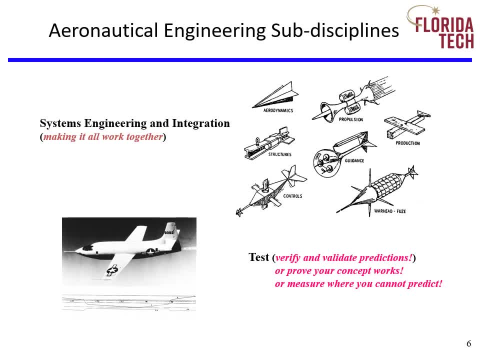 This payload may in turn have its own performance requirements. For example, a radar may have range or angle of attack. The aircraft may also be able to carry a payload in a particular speed, altitude and maneuver envelope over a particular distance. Aircraft performance may also be defined as the ability of the aircraft to carry a payload. 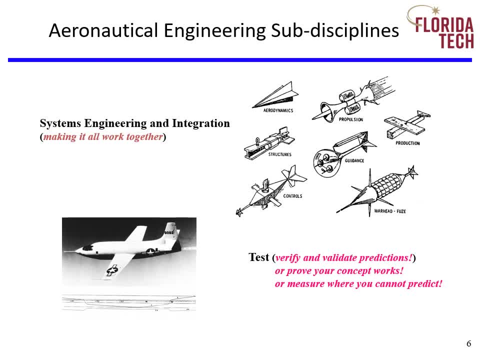 in a particular speed, altitude and maneuver envelope over a particular speed, altitude and maneuver envelope over a particular speed, or even the command of a plane in which it travels. Its ability to place the payload in a desirable operational condition is the entire reason. 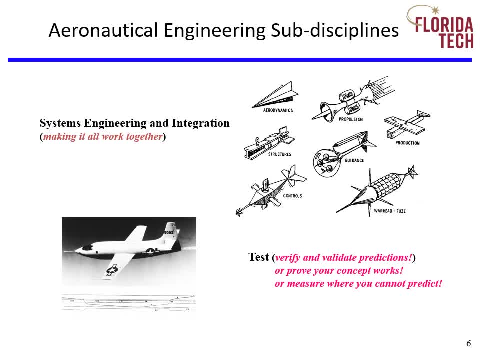 for existence of an aircraft, Systems, engineering and integration is making it all work together. Mission effectiveness of the whole aircraft is some combination of aircraft performance and payload performance, and how well the two are integrated together. All this will be reflected in the output of the actual aircraft, and this is another. way of thinking about the way aircraft performance will be interpreted. 度. I hope this will be helpful as a way to understand the color, shape and weather of a small plane. Thank you for watching today's video. I hope you enjoyed it. I hope you enjoyed it. 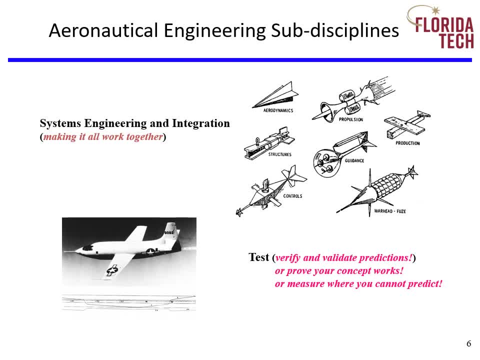 will not have the same as those planned or predicted by the designer. it is essential to quantify where actual performance differs from what the designer intended and the customer desires. herein lies the need for performance flight testing. performance flight testing has been increasingly used to validate aerodynamic and propulsion models used in design validating 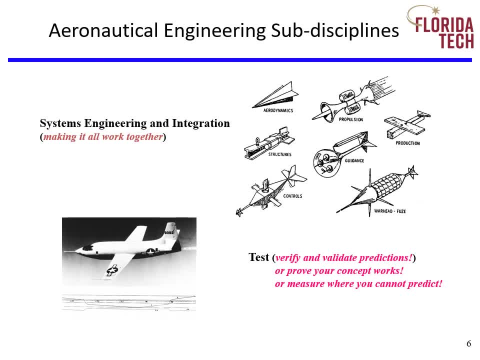 these models greatly reduces performance flight testing requirements, which greatly reduces cost and time required to test new or modified aircraft. once actual performance has been quantified in flight test, the models can be made more accurate, problems in the design can be fixed and insight can be developed for using the aircraft operationally. 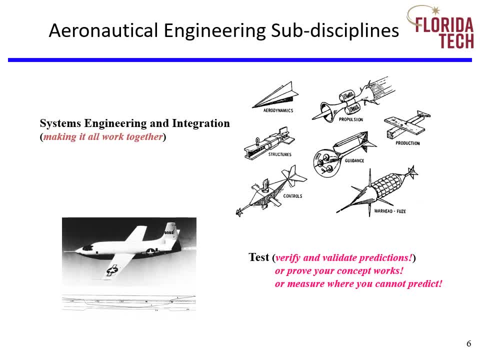 understanding, development, validation and use of aerodynamic and propulsion models is essential to future aircraft performance test programs. performance flight testing can also accomplish several other fundamental purposes: one: determine if the aircraft meets performance specification or requirements defined in the customer statement of need. two: provide data for flight manuals used. 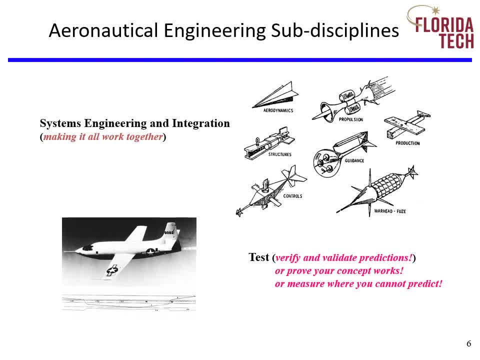 by operational aircrew. three: determine techniques and procedures used by operational aircrew to attain optimum aircraft performance or accommodate adverse performance. and four: obtain data to advance aeronautical science or develop new flight test techniques. operators are usually unconcerned with details of how forces are produced. 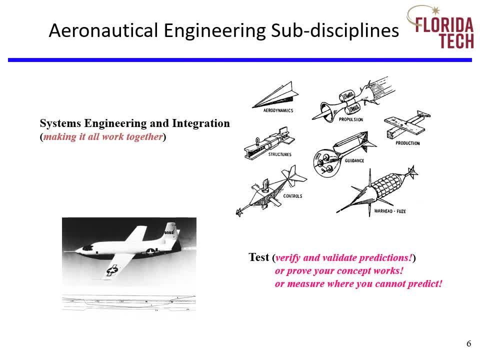 and controlled or how forces are supported. they generally don't care about the details of aircraft design. they also generally are unconcerned about details of obtaining flight design. flight test data, so long as they are confident the test conditions adequately model operational use of the aircraft. They want to know what the aircraft can. 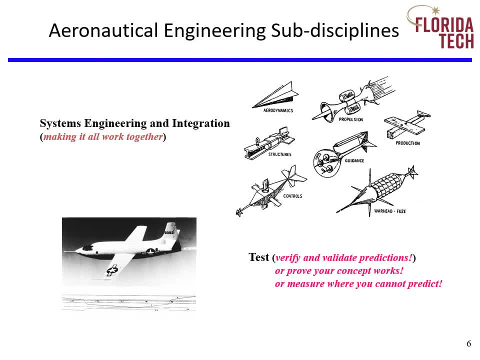 do, how easy it is to fly while using the mission payload or systems, and how much it costs in order to effect decisions about how the aircraft is put together. Unlike operators, flight test pilots, navigators and engineers must be concerned with the details of aircraft design, performance analysis and flight. 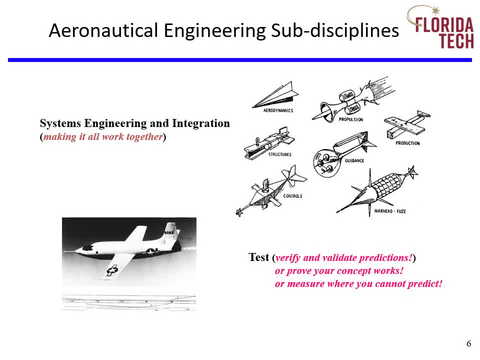 test in order to meet the operators needs for information about their aircraft. As aircraft become more sophisticated, better methods of performance prediction, analysis and testing will be required. Experimental test pilots, navigators and flight test engineers must lead in developing these tools. The material in this course provides a foundation for the 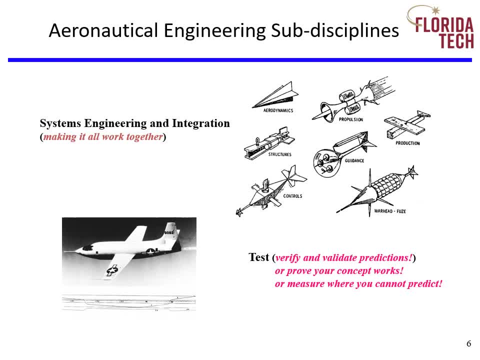 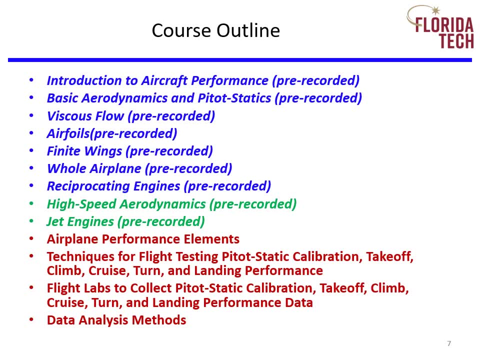 competence needed to be a pilot. This is a hybrid course where the basic theoretical concepts are delivered in pre-recorded lectures and the face-to-face live instruction covers airplane performance elements, flight test techniques, flight labs and data analysis methods. We'll use tools learned in college dynamics courses to calculate performance. 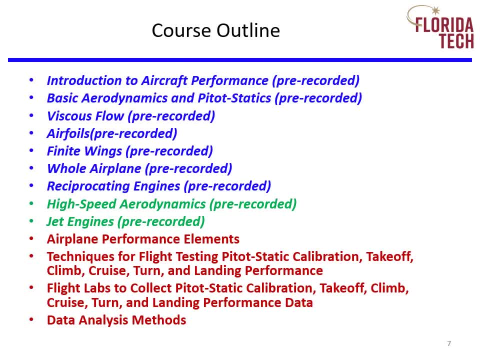 perspective and performance. This simple description of calculating performance is a little misleading, because aerodynamics, propulsion and dynamics are tough problems. The only way to solve them is to break them down into manageable pieces, do the small calculations, reassemble the results back into the whole picture and hope nothing got. 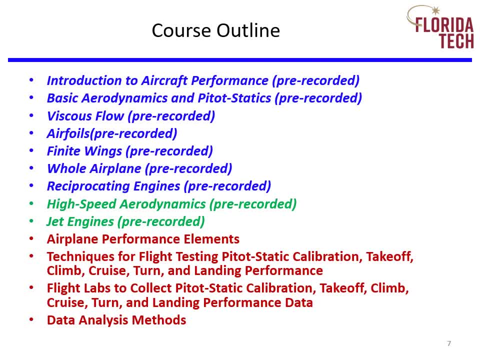 left out along the way. This can be a long road and a map is essential to keep the big picture in mind. The formulation of the complete governing equations for fluid motion and the a motion for solid bodies can be daunting to students Once the equations are developed. 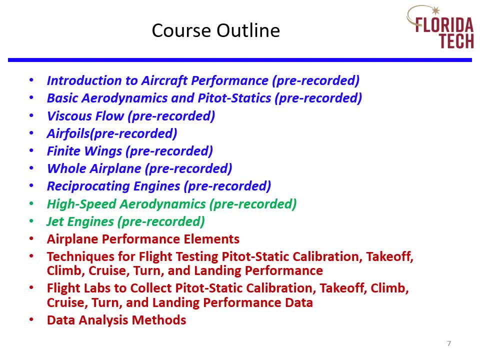 they must be simplified to be solved. This simplification is distinctly different from formulating the governing equations. Simplifying the equations also seems complex to students if they do not know where they are in the big picture or if they do not take the time to appreciate the physical meaning and appropriateness of the assumptions. 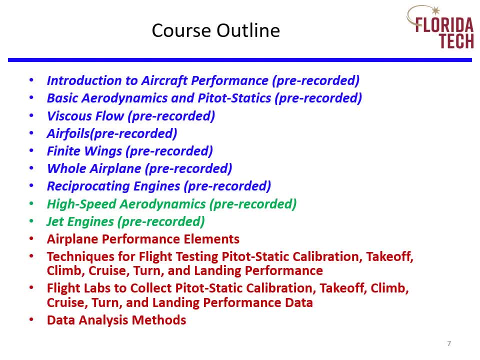 This appreciation includes why the simplifying equations work and what limitations they impose on the solutions when they are applied to real problems. In many cases, students are hopelessly lost by the time the equations are solved, and the most important part of the course- solving these equations- to find forces- is therefore lost on the students. 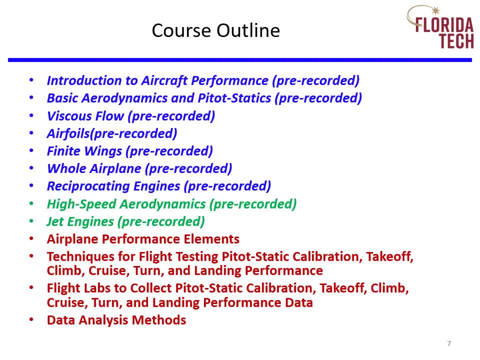 Using pre-recorded lectures that can be rewound is an attempt to prevent that tragedy. The objective of this course is to understand how the sum of the forces affects motion of the aircraft along its trajectory and how the aircraft gains and loses energy In this course. 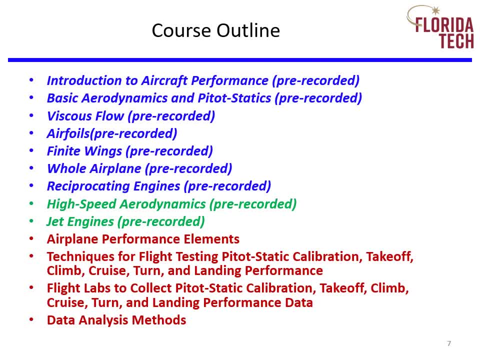 once total force and mass are known, Newton's second law can be simplified to an algebraic equation and solved directly. to yield insight about the forces acting on the aircraft and the motion created by those forces, Energy state can be calculated directly from the equation. 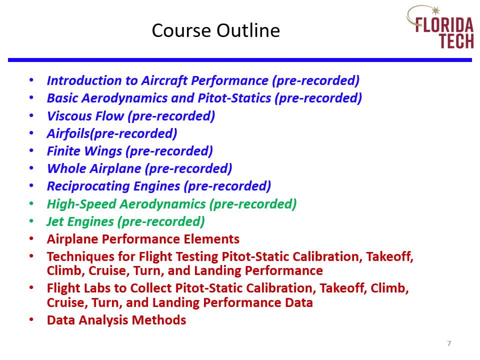 In other words, the force that is given to the aircraft when it is in motion is directly used in the operation of the aircraft. This description of aircraft motion completely describes aircraft performance and provides simple rule-of-thumb type models that answer questions like how well can the aircraft accelerate or climb, how far or how long will the aircraft 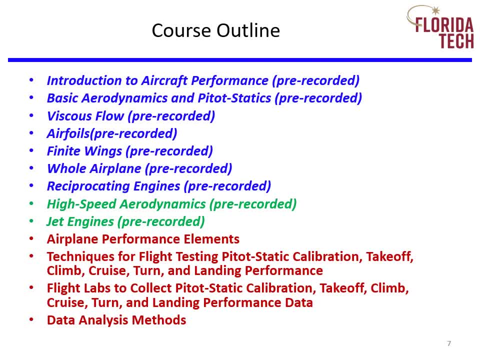 fly on a load of fuel? what length of runway is required for takeoff and landing? What's the aircraft's maximum sustained turn rate? applications requiring very precise information, for example flight simulation, flight control systems, tracking algorithms may subsequently integrate acceleration numerically with respect. 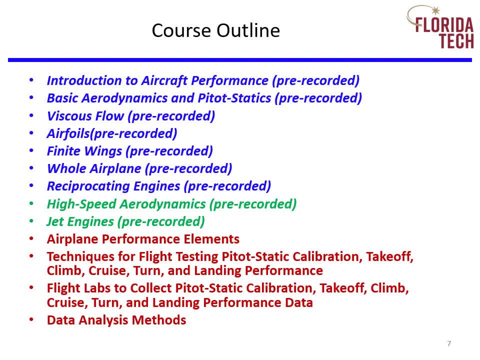 to time to get velocity and position, and integrate with respect to path to get trajectory. Performance is simply the application of dynamics to the result of aerodynamics and propulsion. This type of analysis is essential to virtually all engineering for things that move. It also explains why dynamics is taught rigorously to undergraduate engineers and students. 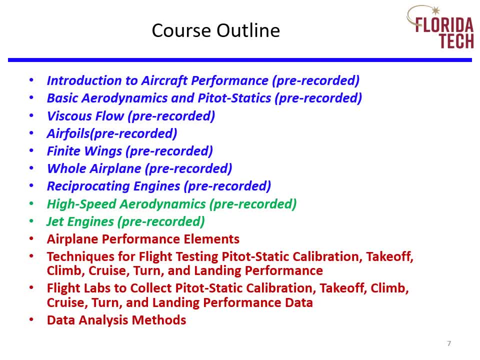 and the skill and the basics of dynamics is essential for flight testers. I recommend reviewing the pre-recorded lectures before starting the face-to-face instruction. but if you're not able to get through all of them, that's fine. You'll learn how to do it in a few minutes. 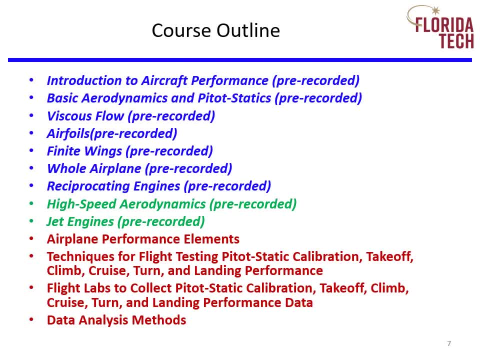 You'll still be able to fly the labs, record and analyze the data. The exam, however, will have questions on the content of the pre-recorded lectures, but only those lectures shown in blue up through reciprocating engines. The exam will not include questions on high-speed aerodynamics or jet engines.